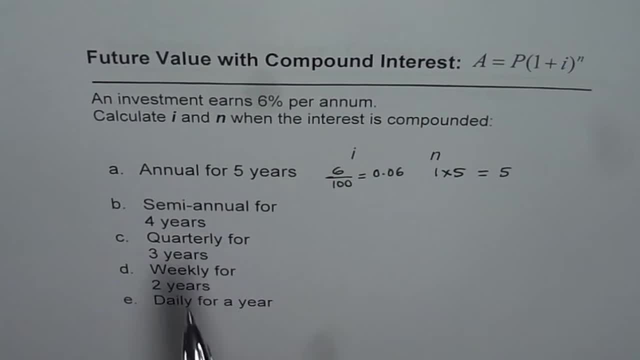 Right Now let's look into the next option, in which investment earns 6% per annum and is compounded semi-annually For 4 years. Now, when we say semi-annually, then it means twice a year. So this interest rate, which is 6% per annum, should be divided by 2.. So what we get here to calculate, I, is 6%. that means 6%, and then you have to divide this by 2, or I could multiply the denominator by 2 times 1 over 2.. So that becomes your interest rate for each compounding period. 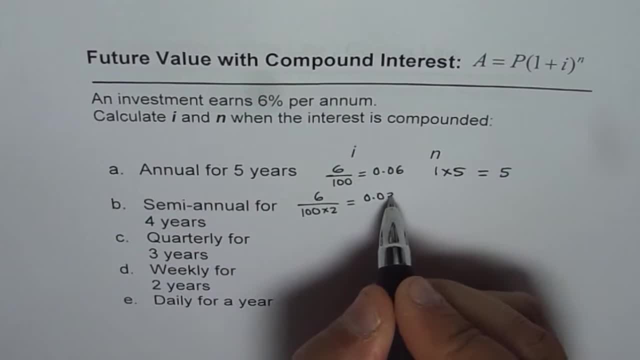 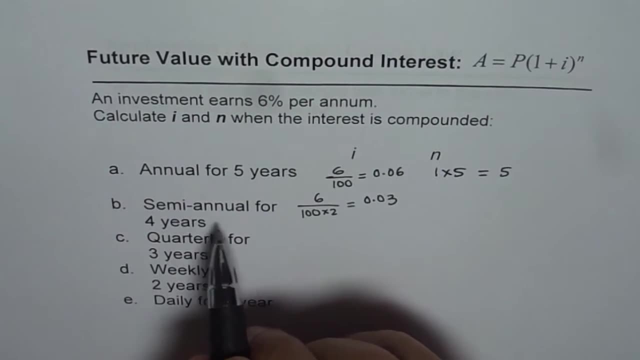 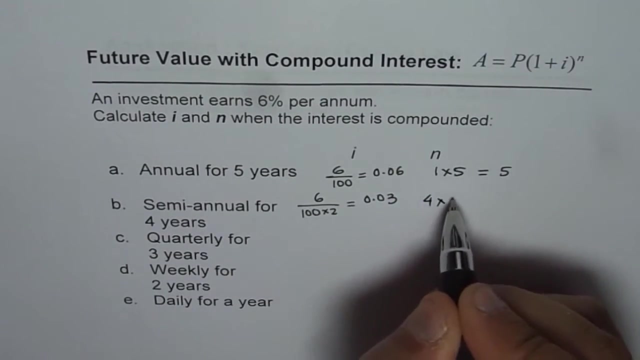 So that means it will be 0.03.. So that is decimal value of the interest rate when it is compounded semi-annually for 4 years. 4 years is number of terms. Now 4 years means 4 years and every year twice. then 4 times 2 gives us 8.. So n value is 8 for us. 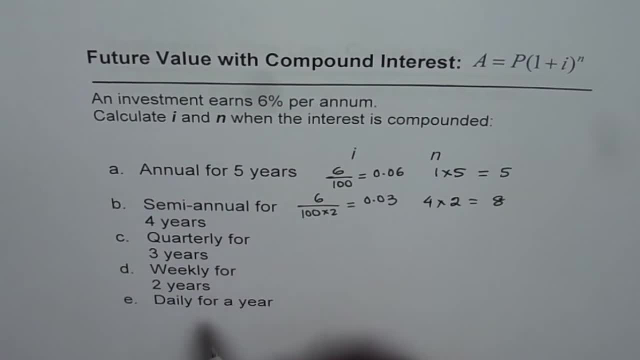 two, because every year it is going to be compounded twice. part C is investment on six percent per annum compounded quarterly for three years. quarterly means you have to divide this by four. six percent per annum, that means six percent six over hundred. quarterly means one-fourth of this right, so you do one. 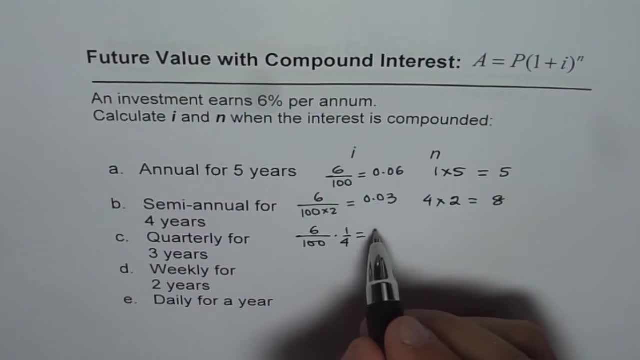 fourth of this one fourth will be zero point. half of this right one, five. let me write right. normally you should use calculator, calculate these values quarterly for three years. that means every year four times. so the value of n is twelve. okay, so that is how we have to calculate the values of I and n, right? so? 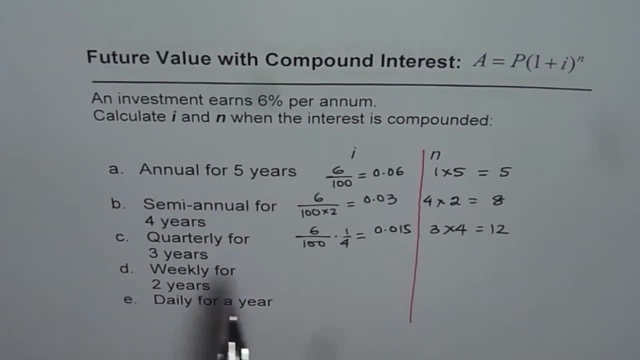 I hope that's absolutely clear now. the next one is when it is compounded weekly for two years. weekly there are 52 weeks in a year, so we'll divide this six over hundred, six percent times three, and then we take that two percent in two years and then we multiply it by the n times. we get the second percent of the. 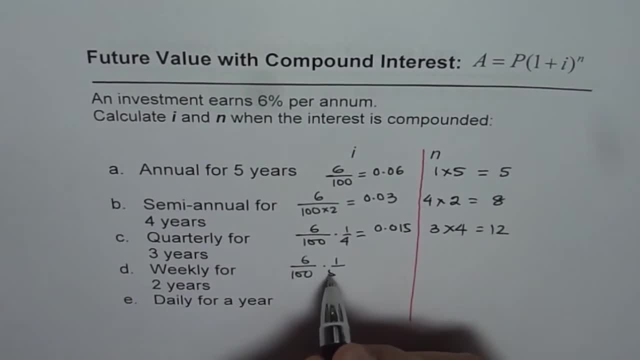 percent per annum by number of weeks, which is 52. so that will be 1.06 divided by 52 and that gives us 0 point. or let me write the fraction value itself, which is better. we will use 3 over 2600, which is kind of simplified form of this fraction, right? so we will use.